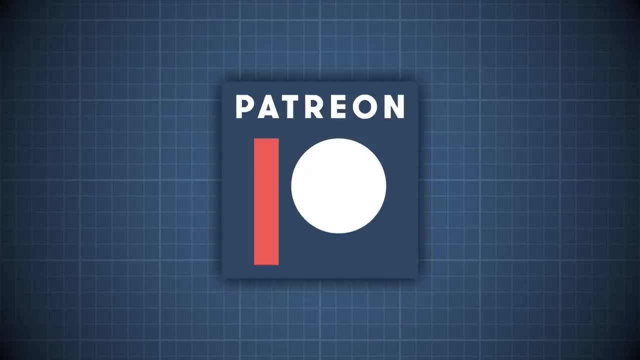 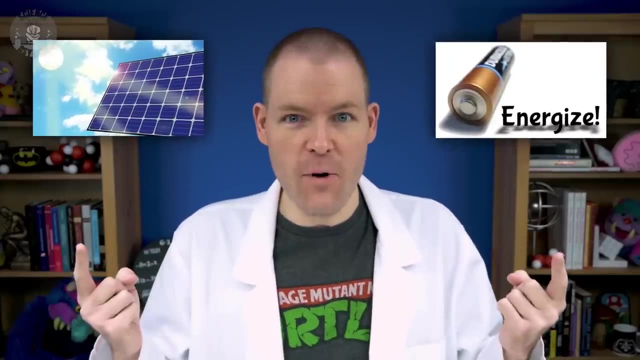 This episode was made possible by generous supporters on Patreon. Hey Crazies, I've done a video on solar panels and I've done a video on batteries, but neither of these methods is how we generate most of our power. So how do we generate most of our power? 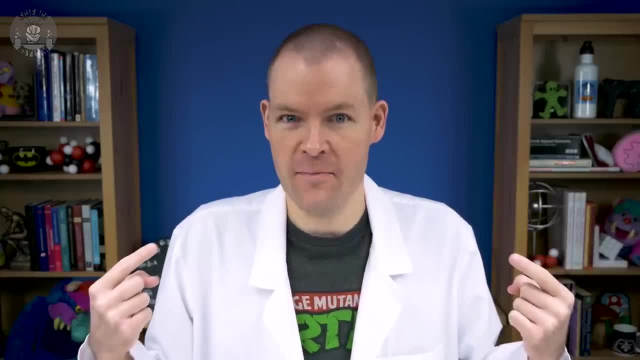 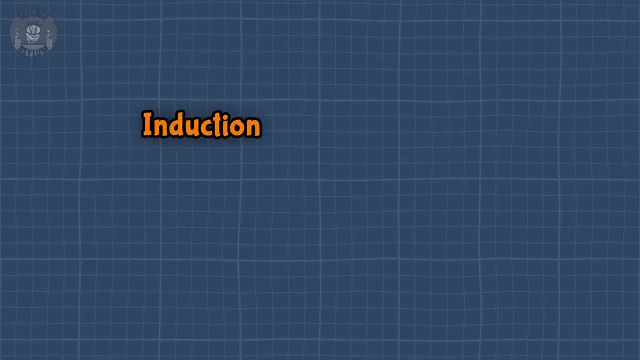 Magnetic induction. I've wanted to make this video for a long time. Let's do this. It seems natural to start with the name magnetic induction. The word induction comes from the root word induce, which just means to cause something by persuasion or influence. 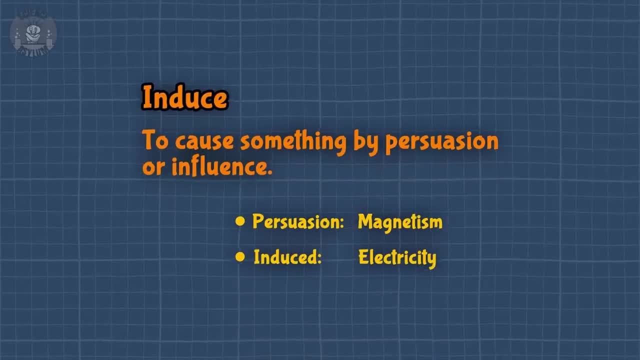 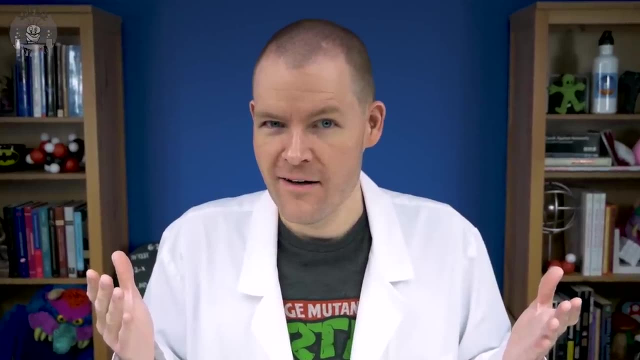 In this case magnetism induces electricity. This method of generating electricity isn't anything new. I mean, it's almost two centuries old To the timeline. All the way back in 1831, Michael Faraday was doing a series of experiments. 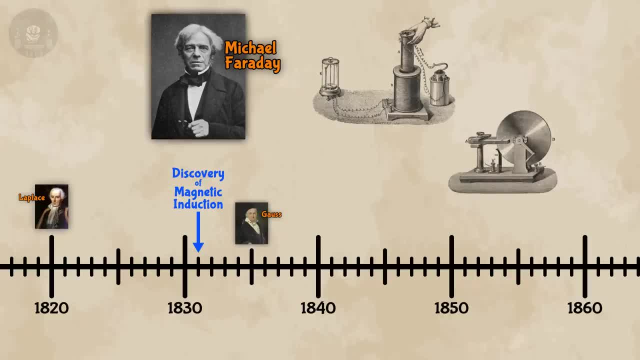 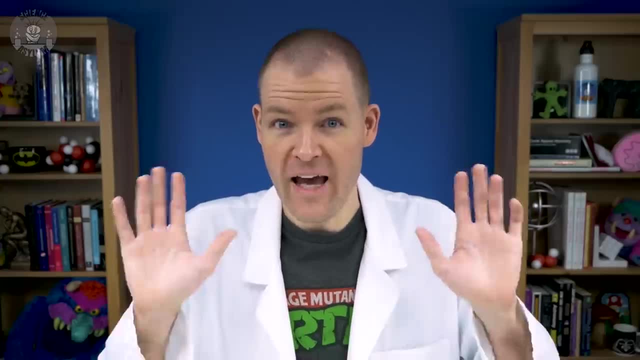 some involving coils and others disks, but I'm getting a bit ahead of myself. We can understand induction with something simpler than a coil. A current in a long straight line will generate a magnetic field. Any moving charge will generate a magnetic field. We call that an electromagnet. 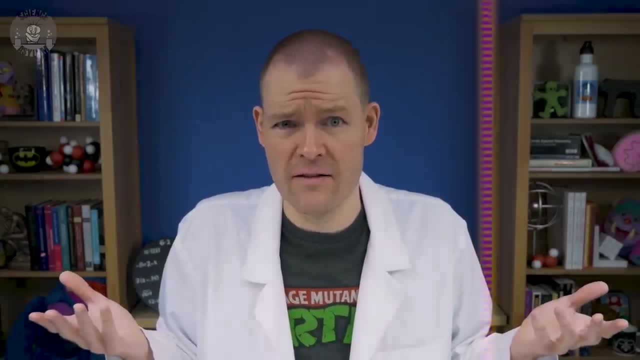 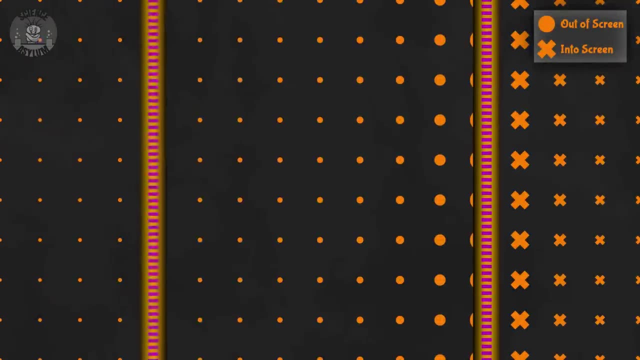 So let's say we've got a long straight wire carrying an electric current. Since current is moving charge, that wire will generate a magnetic field. If there's another wire carrying another current inside of that field, it will be affected by that field. 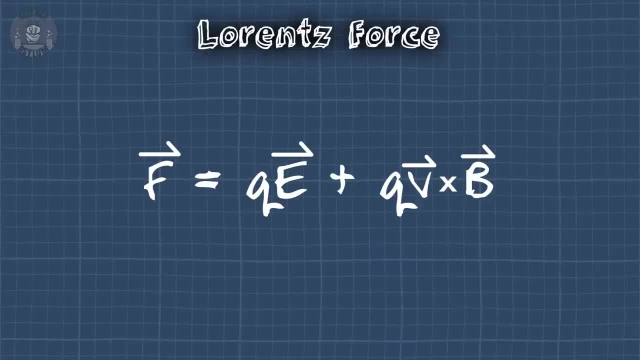 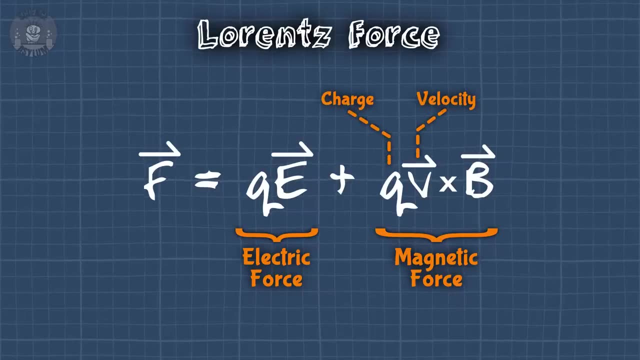 In this case the wire is pushed sideways. That push is a magnetic force, which is part of the electromagnetic force. You can see here. it requires the charge to be moving. Wait, how does all this relate to magnetic induction? Patience Question Clone. 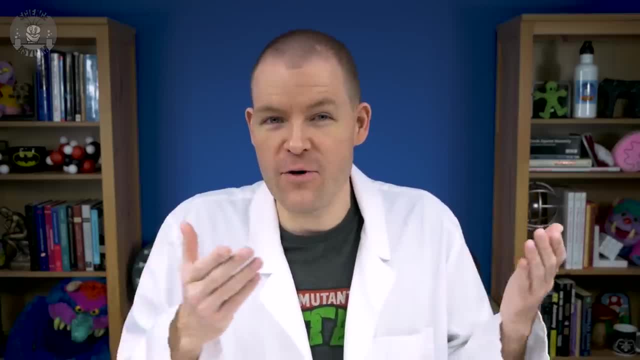 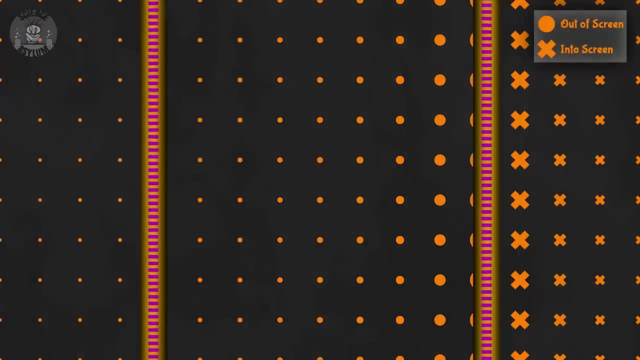 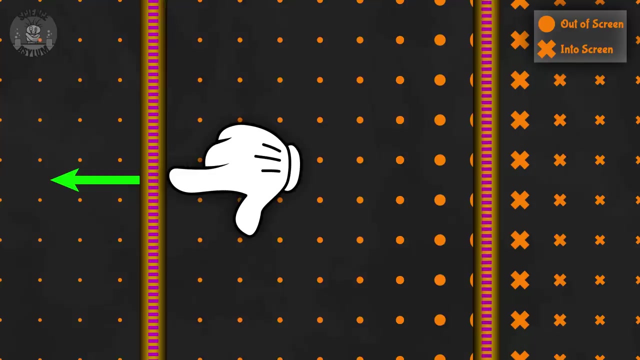 Patience. OK, sure, one current exerts a force on another current using magnetic field. Nothing crazy there. But this process is completely reversible. If the current in a wire can be pushed sideways by a magnetic field, then pushing a wire sideways in a magnetic field should cause a current. 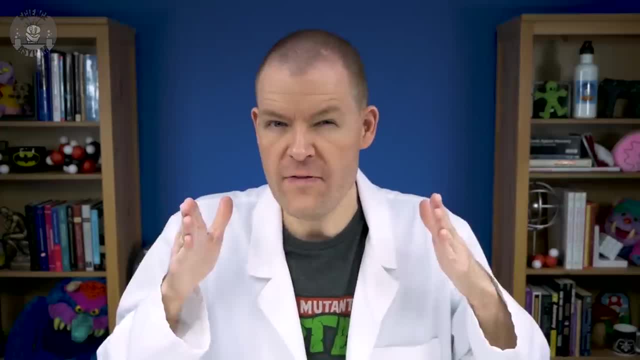 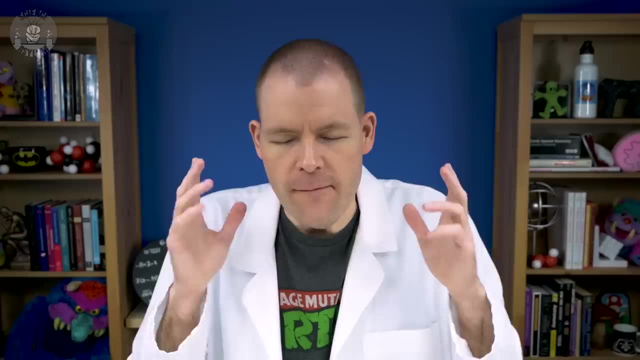 And that's exactly what happens. That's magnetic induction. We've induced a current in a magnetic field through motion in a magnetic field. That's it. Well, yeah, I never said this was complicated. People make this out to be so magical sometimes, but it's just about reversibility. 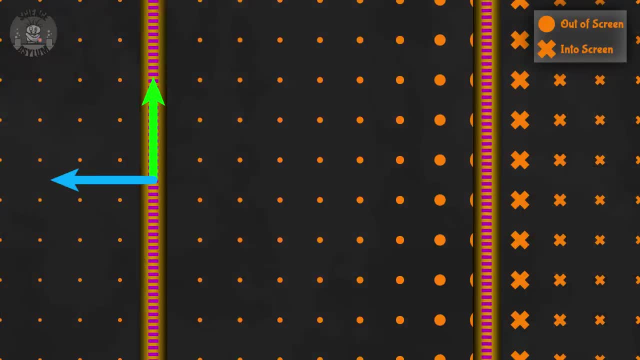 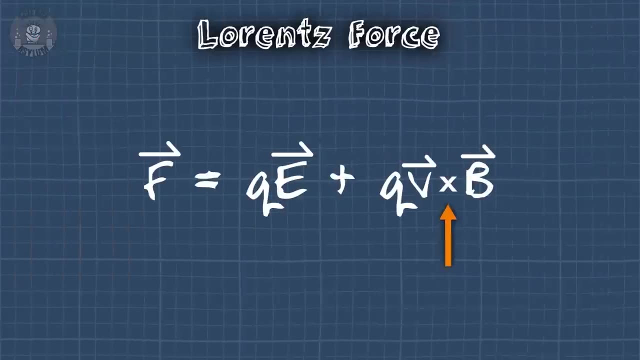 Moving charge in a wire this way gives us an effect. that way All we've done with induction is swap the arrows. We've moved the wire sideways to push the current along. They have to be perpendicular because cross products. But the cool thing is it doesn't even matter which wire you move. 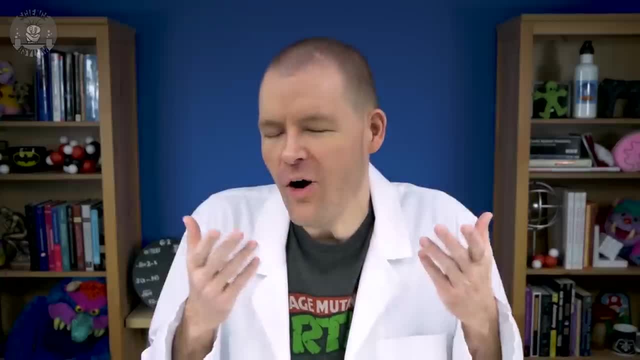 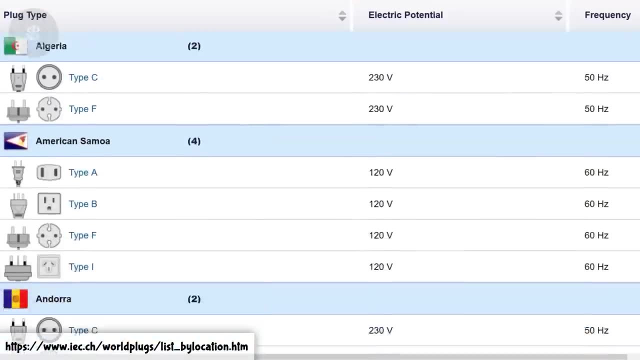 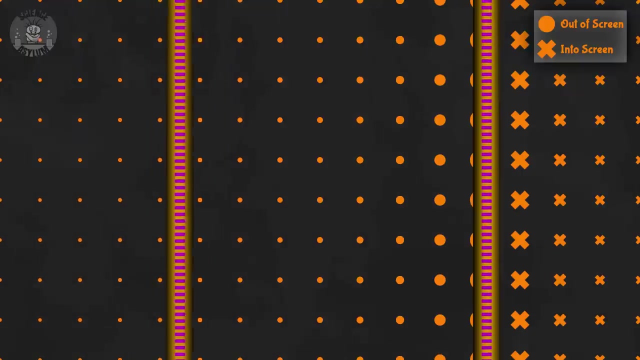 A current will be induced in the second wire regardless. While this setup gives us a simple understanding of induction, unfortunately it's not very practical. AC wall sockets almost always operate at 50 to 60 Hz. That means I'd have to wiggle this wire back and forth 50 to 60 times per second. 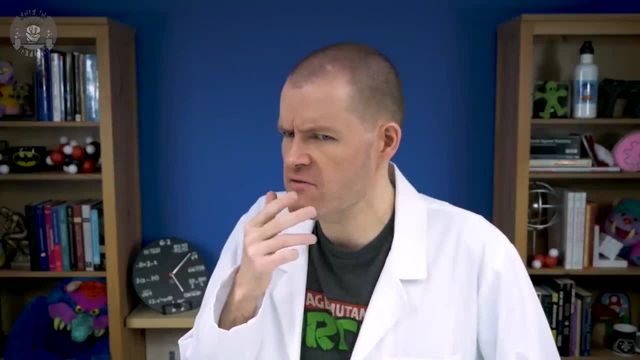 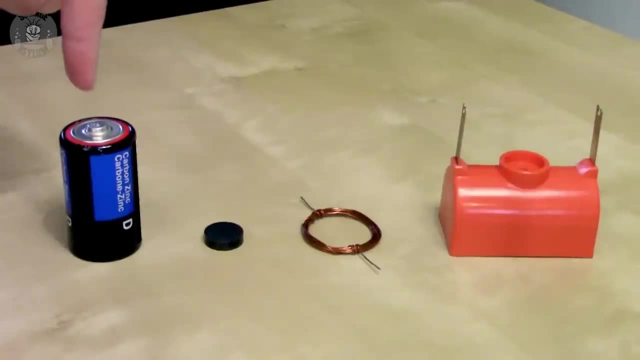 which is kind of ridiculous. Hmm, what's something else that cycles that we can reverse? What about an electric motor? You know that might actually work. We can build a simple motor using a battery, a magnet, some insulated wire and a few other things, just to hold it all together. 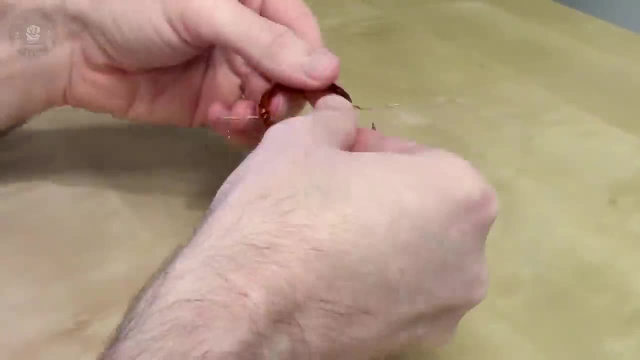 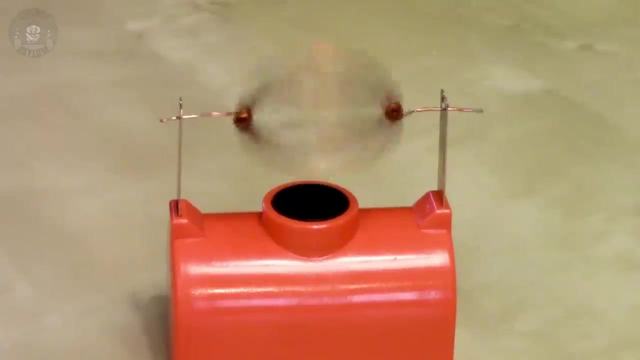 You wrap the wire into a coil and set it up, so current will run through it. All it needs is a little nudge to get started and it'll spin as long as it has energy from the battery, Just like the straight wire case. 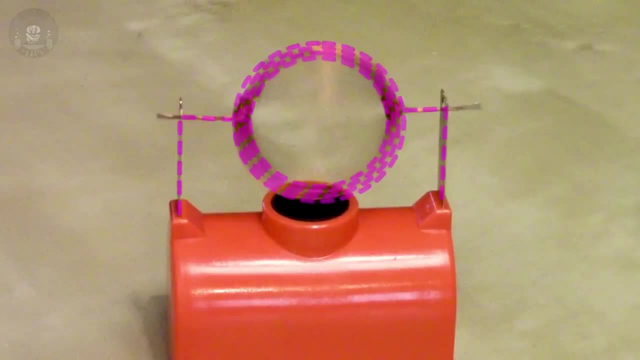 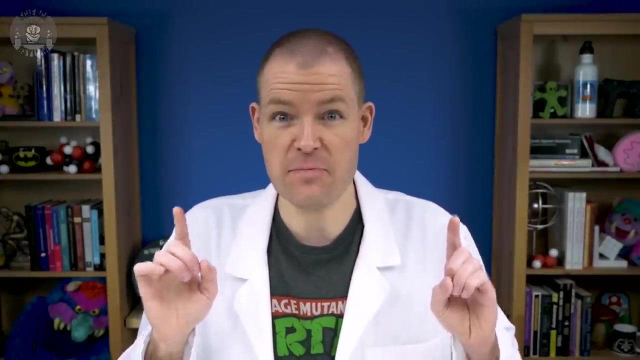 charge is moving through the coil wire inside a magnetic field, so there's a force on it. Now let's put that thing down, flip it and reverse it. It's the server net. It will find me if I don't let it work it. 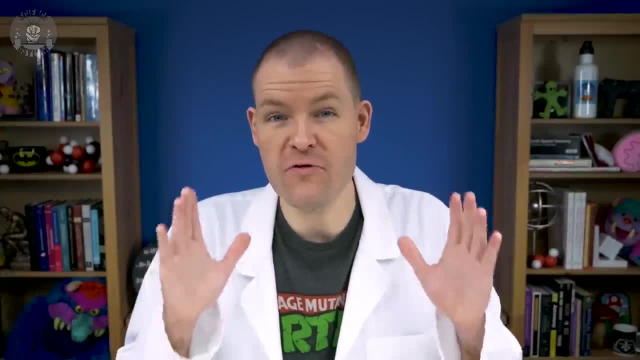 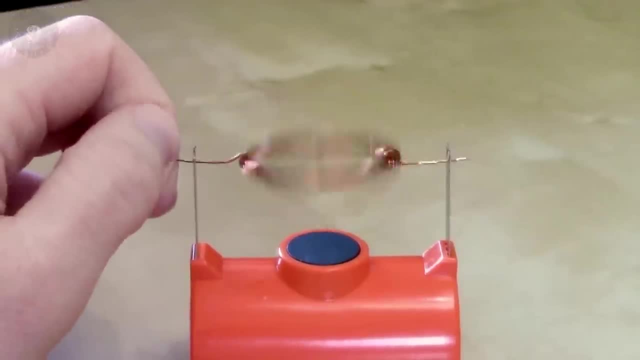 I need a glass of water. Anyway, what happens if we reverse it? We remove the battery and just spin the coil by hand. Doing this should induce a current, just like moving our wire did before. Well, at least if we have somewhere for that current to go. 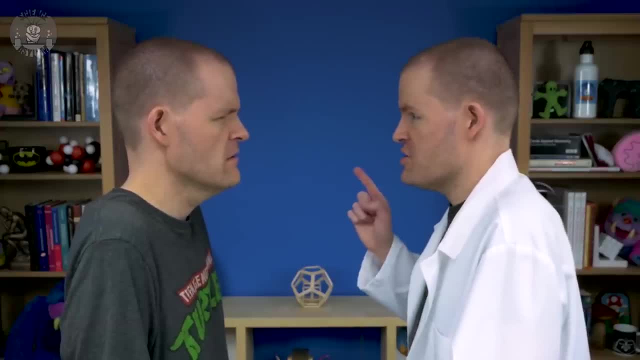 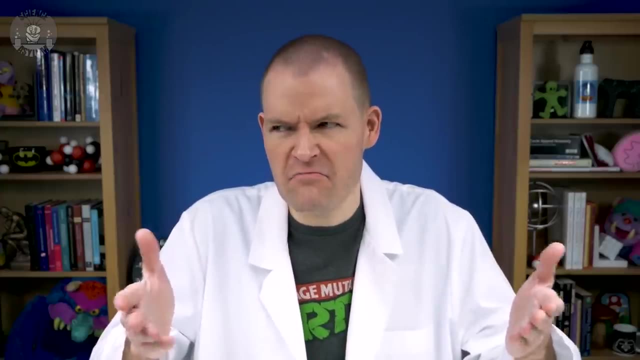 What do you get if it's just sitting there not connected to anything? A voltage, That's just energy per unit charge. It's the energy the charges need to move forward to make a current. if they could, In this case you might not have a current yet. 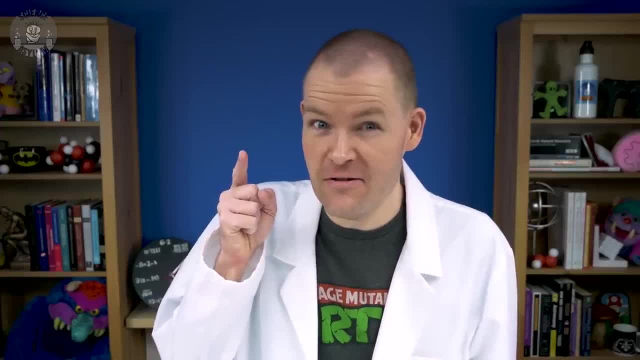 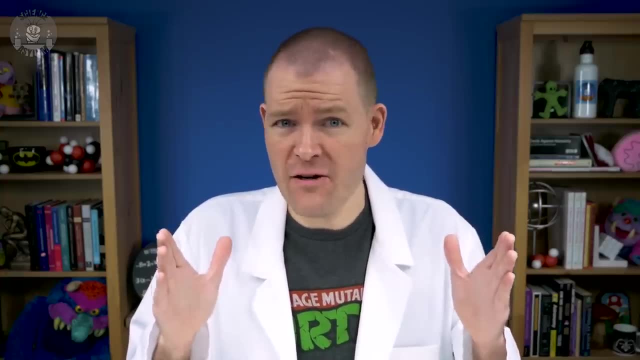 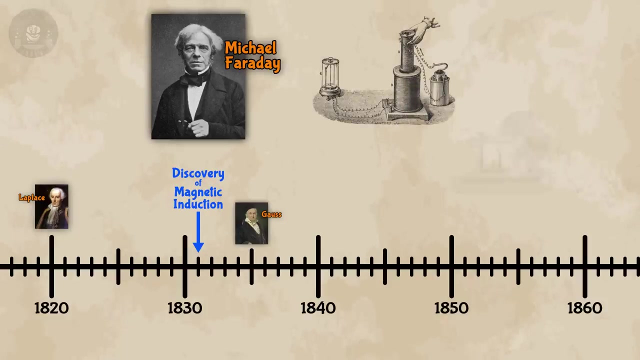 but there's still a potential for one. Get it A potential, Because another name for voltage is electric potential. Never mind, The point is a simple: electric generator is just a backwards motor. Back in 1831, Faraday was generating voltage by moving coils around and spinning disks. 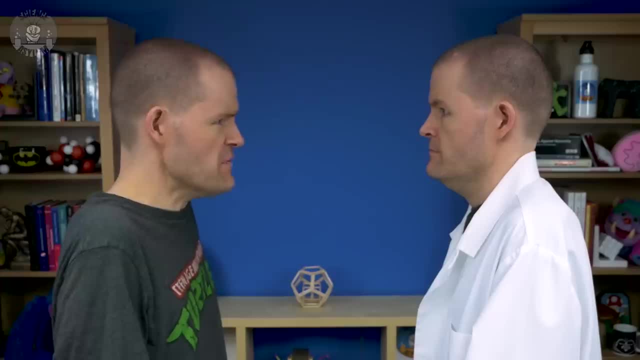 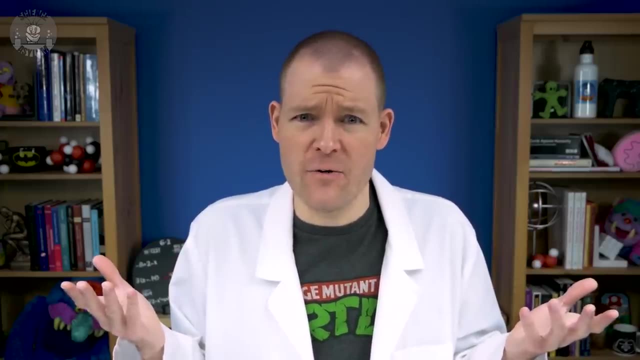 We've just combined those ideas by spinning coils. So how much voltage does it generate? Well, that depends. In order to make predictions about anything physics related, we need an equation. The concepts discovered by Faraday weren't written mathematically. 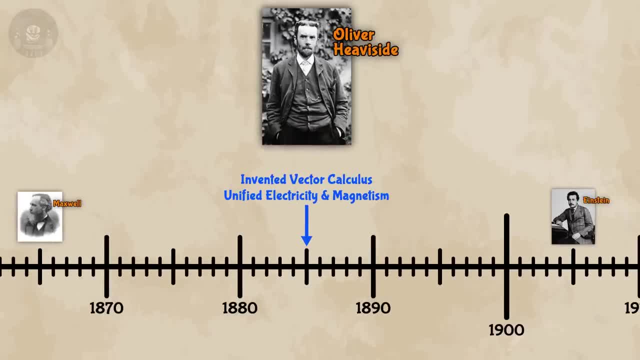 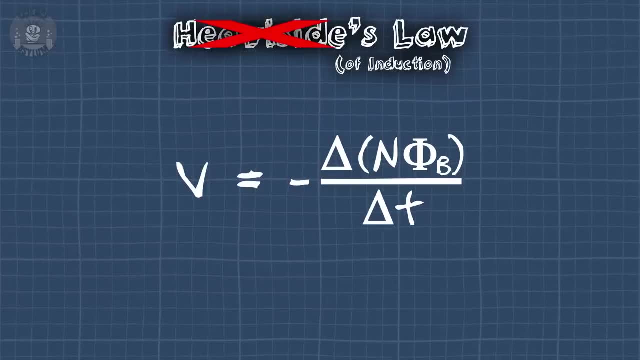 until about 1885, when Oliver Heaviside properly unified electricity and magnetism. That's why the law describing magnetic induction is called Heaviside's Law. Just kidding, It's called Faraday's Law. I'd like to tell you that's because Heaviside already had a bunch of stuff named after him, like Laplace. 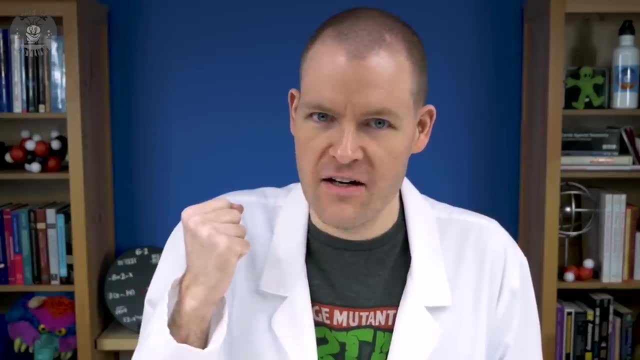 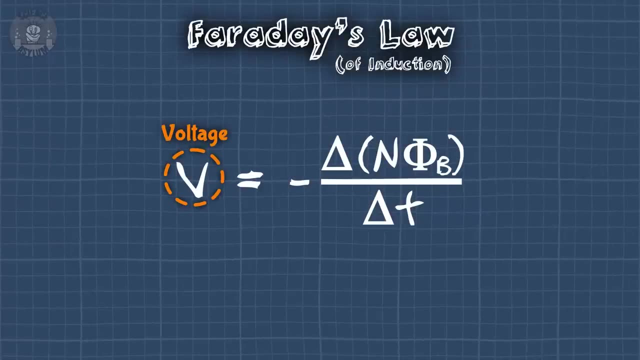 Unfortunately that's not true. Heaviside really got shafted here. But let's try to read Faraday's Law in plain English. On the left, there's the result: we're looking for A voltage. On the right, we've got the cause of it. 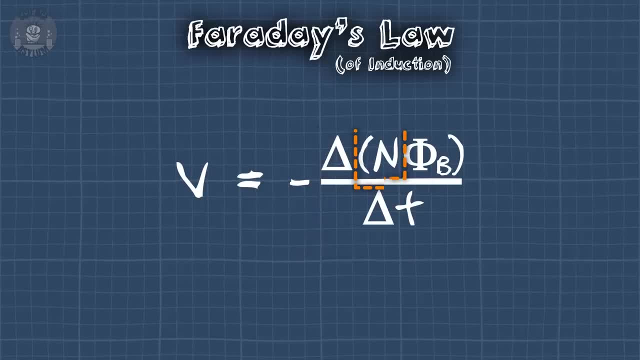 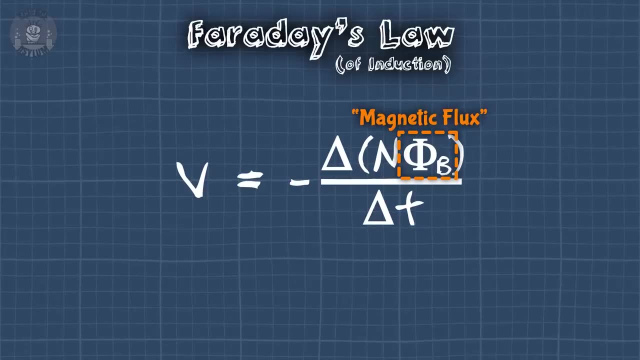 The cause of that voltage? A change over time. The n is just the number of loops in our coil. The phi is the magnetic field on an area Also known as magnetic flux. The fact that it's called flux isn't important though. 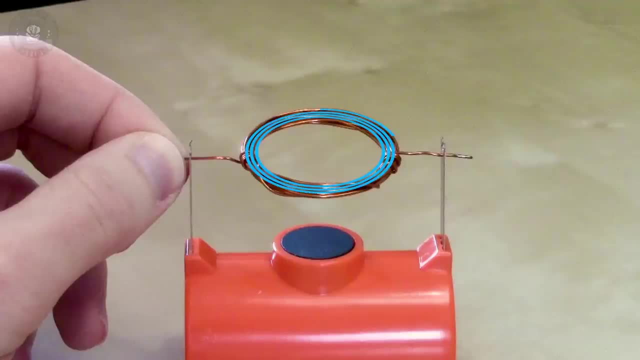 You know what? Forget? I even mentioned it. Our coil has maybe 10 loops in it, So n equals 10. Nice and easy. The coil also forms a circular area, An area that has a magnetic field inside it, The field inside that area. 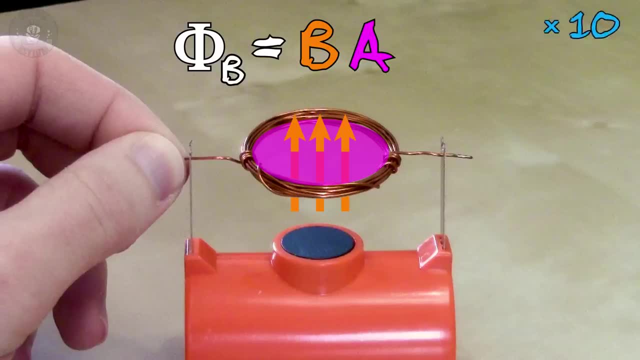 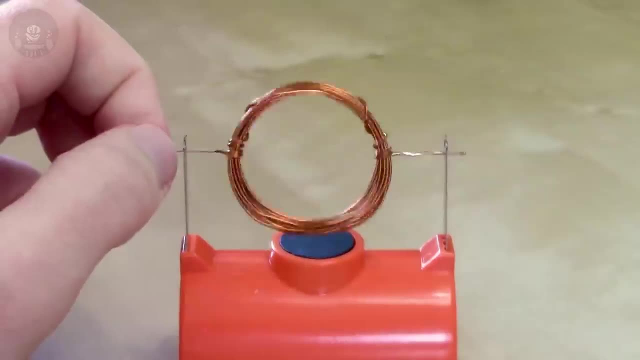 multiplied by the area itself, is that phi symbol. Then we multiply by 10 because there are 10 loops And bam, We've got a number we can use in Faraday's Law. That number changes because the loops are spinning. Sometimes they have a lot of magnetic field inside them. 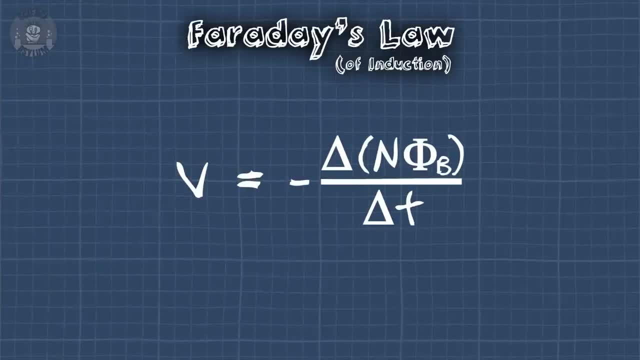 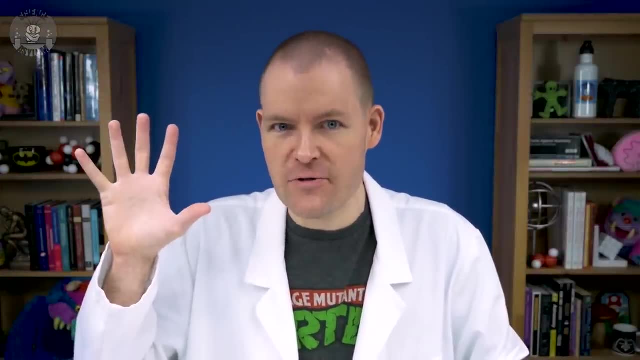 Sometimes only a little bit, Sometimes none, And according to Faraday's Law, that change gives us a voltage. Our backwards motor transforms the energy from my hand into electrical energy. Of course, turning this by hand is a lot of work I'd rather not do. 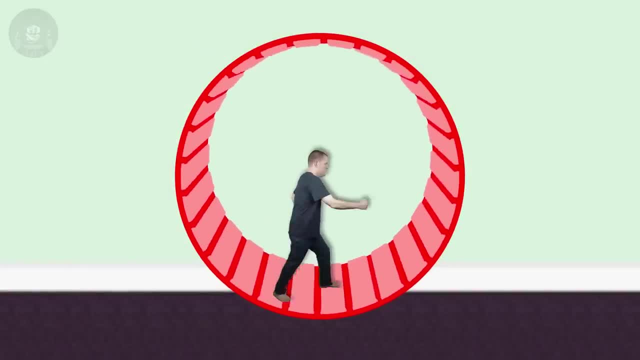 Having hamsters or clones running in wheels would be a lot less work. Having hamsters or clones running in wheels would be a lot less work. Having hamsters or clones running in wheels would be a lot less work, But that's not very scalable. 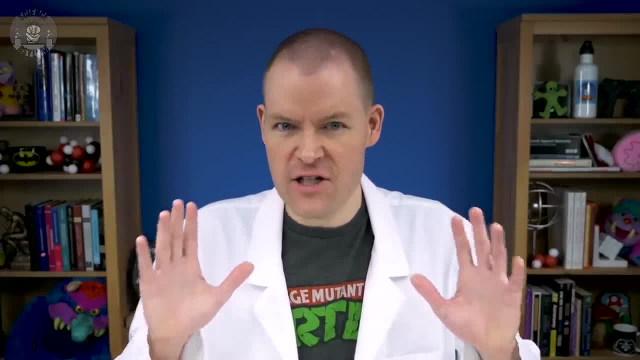 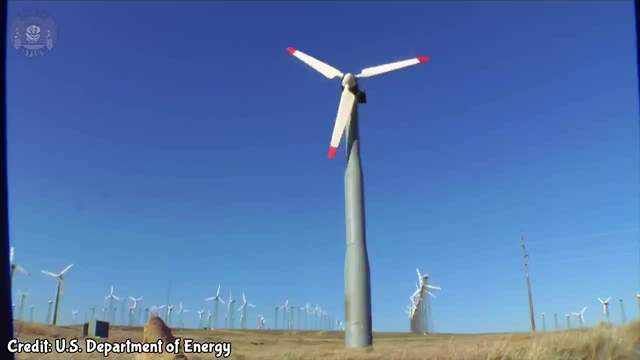 This method might be 200 years old, but we've gotten a lot better at engineering it. So how do we generate most of our power? By making coils spin inside magnetic fields. Wind power: The wind turns the blades which are attached to a coil.